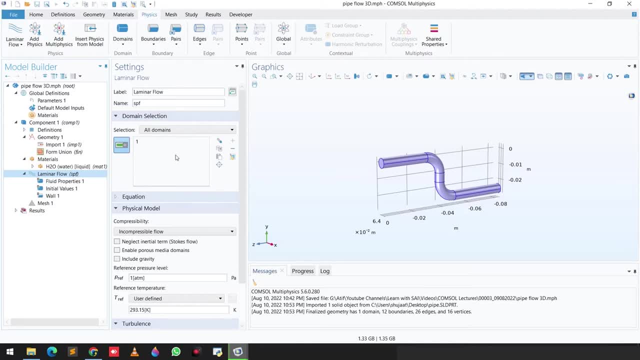 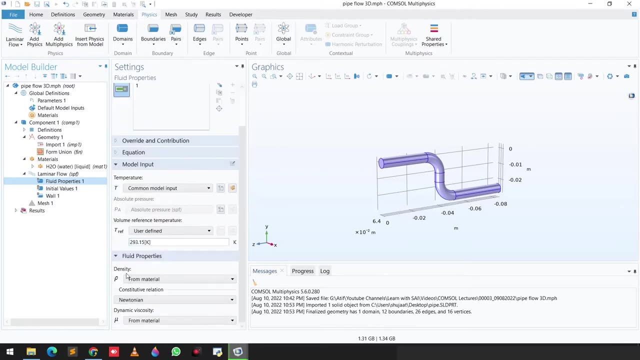 first of all, select this whole domain as a fluid domain. And the next step you need to select that you are going to take the fluid properties from the material. We already are going to do that in the next step, So we will first select the fluid property from the material. 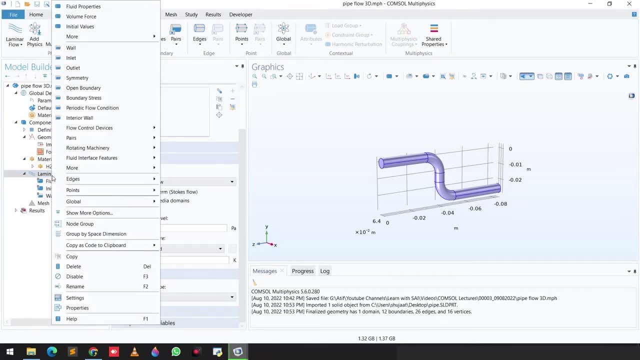 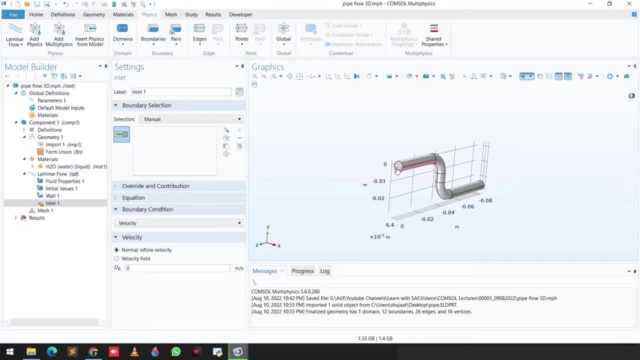 And, as you can see, here the fluid property is assigned. So that means that the fluid is assigned here And now we have to add some input and output values, like where the fluid will go in and out, So inlet and outlet values. So for the inlet, I am going to select this one as an inlet. 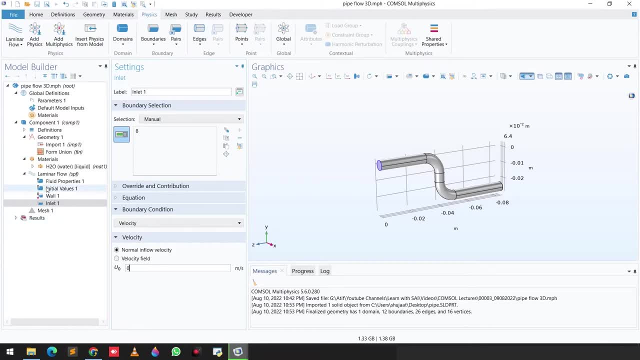 And I'm going to add the velocity. So I'll tell you that how we can add velocity. I will define a function, Then I will solve the inlet velocity for that function. So in the next step you need to click here and select that. 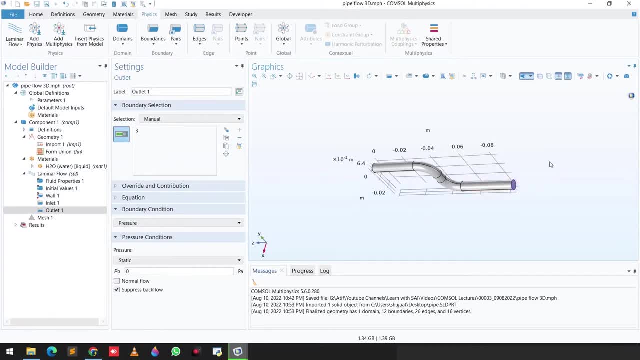 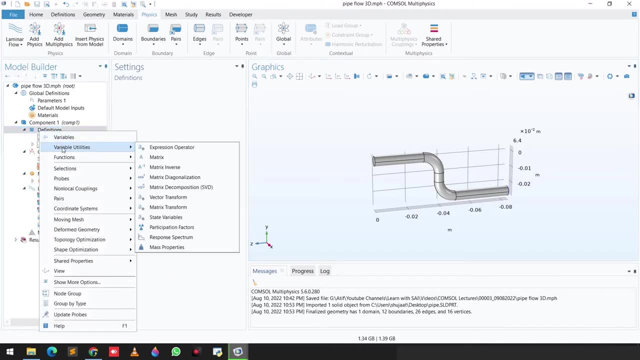 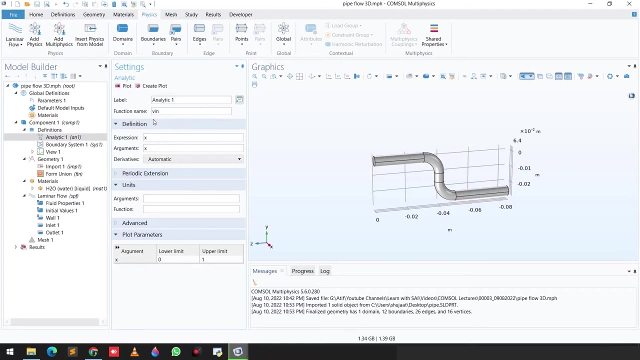 select the outlet. this will be our outlet. so we need to define a velocity function. so we'll go to the definition and right click on that and add a function here and this we will say this is V. in is the inlet function, and we will define the function value. we'll say it 5. 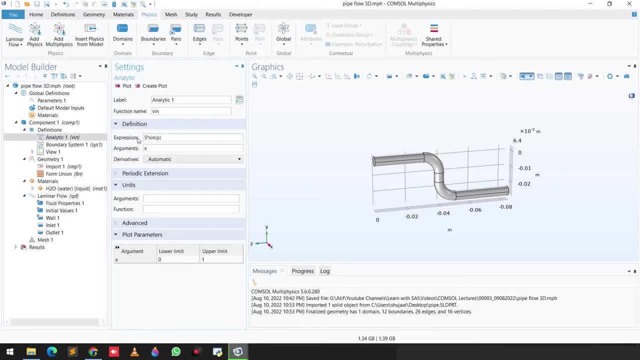 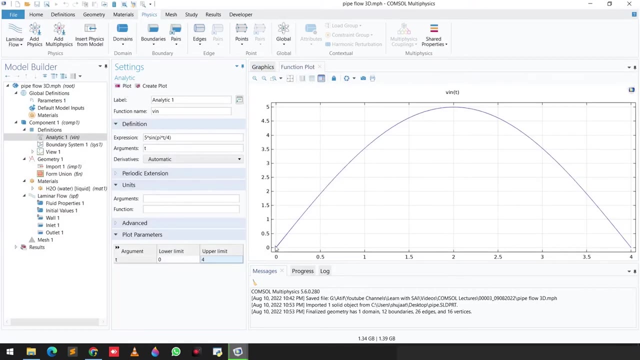 multiplied by sine of pi into T divided by 4, and the argument is T and we are going to solve it for 4 and then you can see here the velocity function. so velocity function will go from 0 to 5 meter per second and then it will come back again. 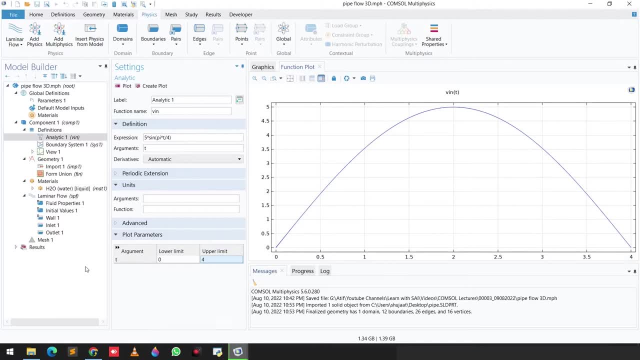 to 0 when the time is 4 seconds. so we are going to add this function. you can add the units here for the argument and the function. so click here. for the argument, we are going to say it's in second, and for the function we can say it's meter per second. so we'll go to the. so we'll go to. 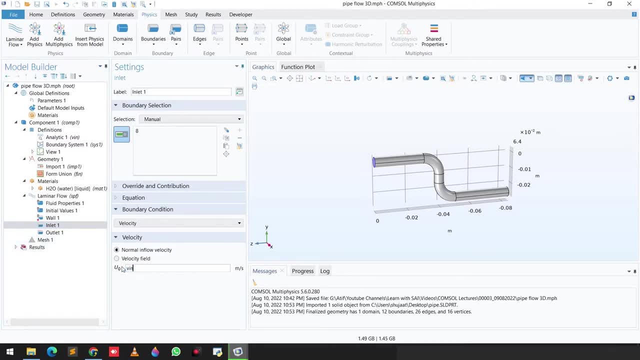 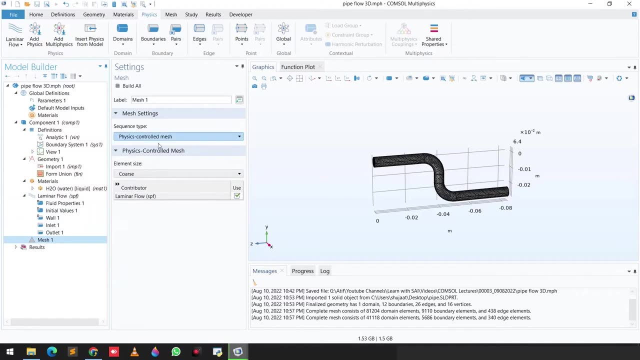 the inlet and then we will assign this function as an. so in the next step we will go to the mesh. as you can see here, this is a physics controlled mesh, and this is a physics controlled mesh and element size will be coarse. so this is element size will be coarse. so this is already developed. so to make the 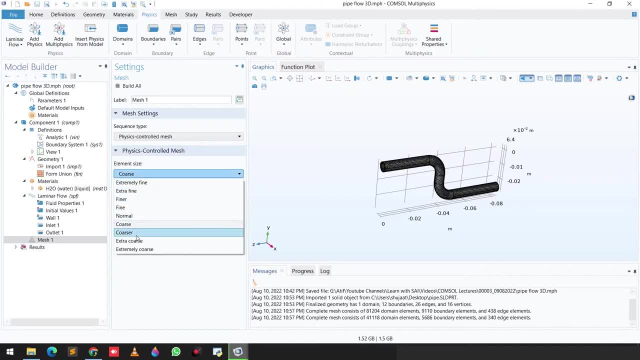 already developed. so to make the simulation quicker, we will go for coarser simulation. quicker we will go for coarser mesh. select the coarser mesh and then mesh. select the coarser mesh and then click the build. click the build and now you can see here the mesh, the 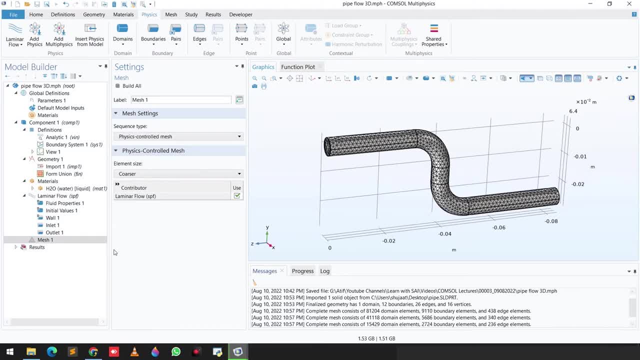 and now you can see here the mesh. the coarser mesh has been generated. so the coarser mesh has been generated. so the next step: we have to select the study. so next step, we have to select the study. so go to the study step and then add a. 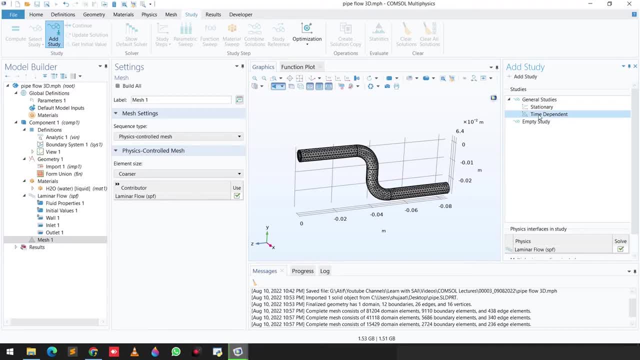 go to the study step and then add a study. so we are going to perform time study. so we are going to perform time study. so we are going to perform time dependent study. click on the time dependent study. click on the time dependent study, click on the time dependent and we have time dependent. 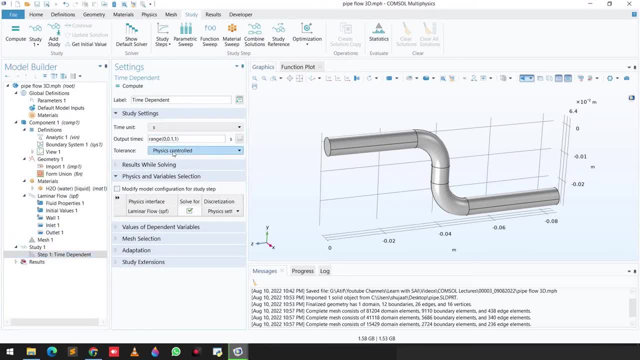 dependent and we have time dependent, dependent and we have time dependent. study here. so we are solving our problem. study here. so we are solving our problem. study here. so we are solving our problem for 4 second with 0.2 time step and we for 4 second with 0.2 time step and we. 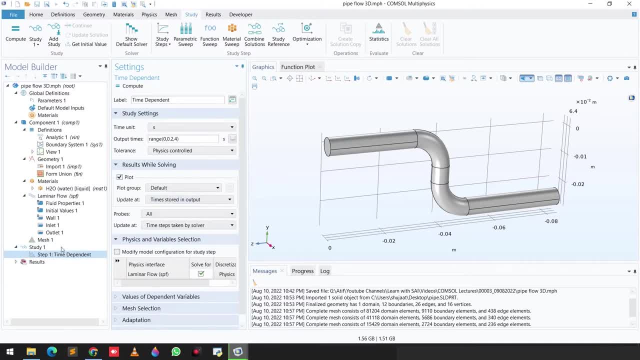 for 4 second with 0.2 time step, and we want to see the result while it's want to see the result while it's want to see the result while it's solving. so that's all, once you are done solving. so that's all once you are done. 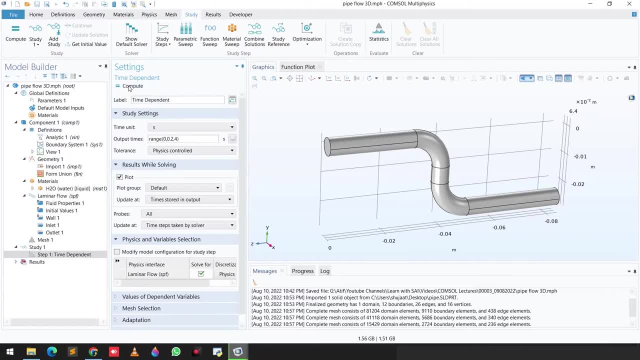 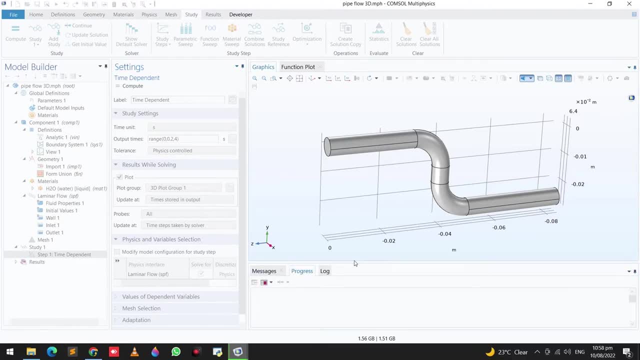 solving. so that's all. once you are done, just click on the compute button. just click on the compute button. just click on the compute button and the simulation will start. and the simulation will start. and the simulation will start. you can see here: this is the function input. 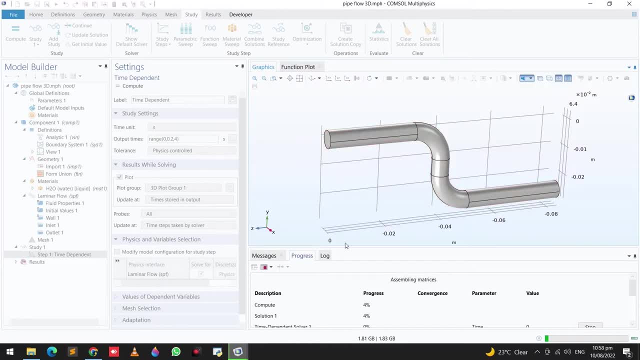 you can see here: this is the function input. you can see here this is the function input. velocity function. we have plotted velocity function. we have plotted velocity function. we have plotted and you can see here the simulation has. and you can see here the simulation has and you can see here the simulation has been started. now it's 4% done and in a 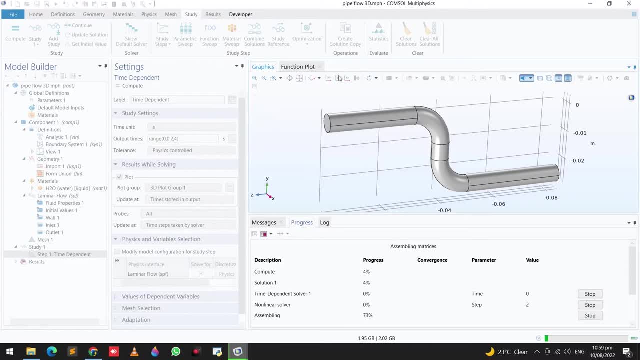 been started, now it's 4% done. and in a been started, now it's 4% done. and in a few second we will get the merges plot. few second we will get the merges plot. few second. we will get the merges plot here and you can click and see how your 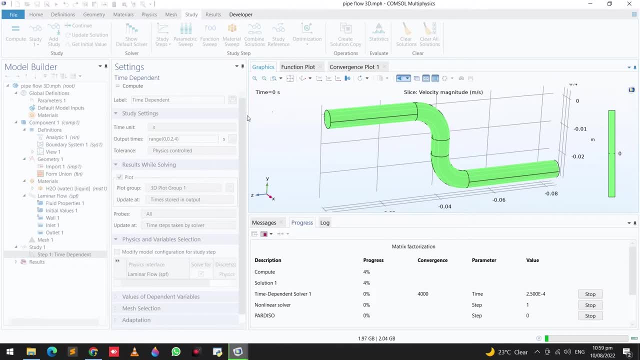 here and you can click and see how your here and you can click and see how your simulation is in process. so you can see simulation is in process. so you can see simulation is in process. so you can see, here, as we selected, this result, while here, as we selected this result, while. 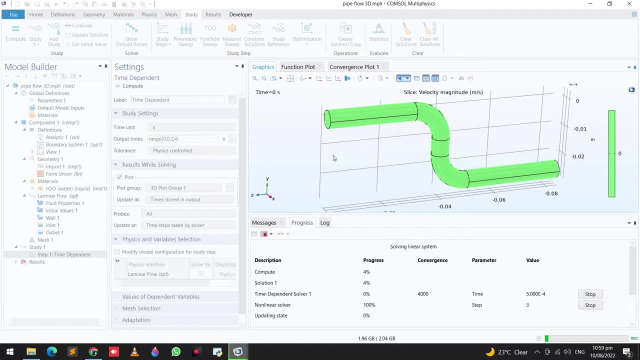 here, as we selected this result while solving conditions. so we can see the solving conditions. so we can see the solving conditions. so we can see the results while it's being solved. so you results while it's being solved. so you results while it's being solved. so you can see here as well, we have, we got the. 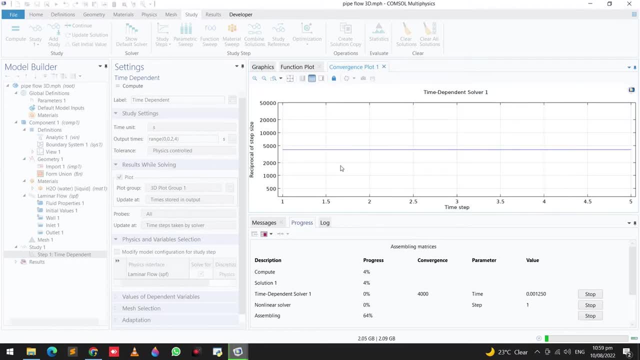 can see here as well, we have. we got the can see here as well, we have. we got the convergence plot so you can monitor the convergence plot. so you can monitor the convergence plot, so you can monitor the progress of your simulation here, so it progress of your simulation here, so it. 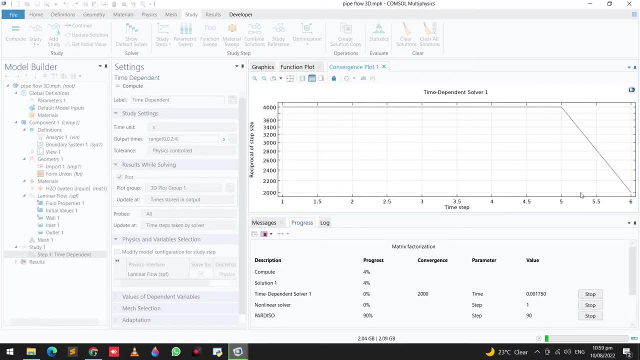 progress of your simulation here. so it should go down and it should the error should go down and it should the error should go down and it should the error should reduce when we approach more time, should reduce when we approach more time, should reduce when we approach more time steps. so if you can go here and you can, 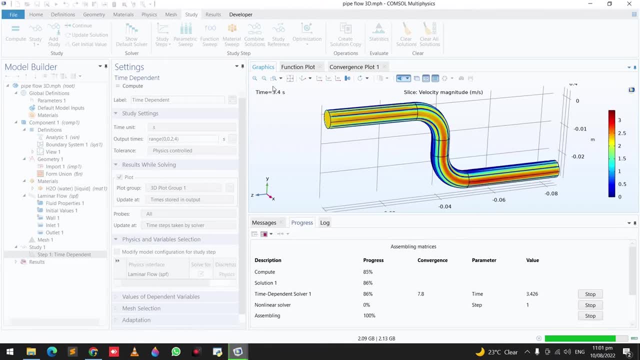 steps. so if you can go here and you can see it's in process, as you can see here, see it's in process, as you can see here, see it's in process, as you can see here- that we already solved for 3.4 second, that we already solved for 3.4 second. 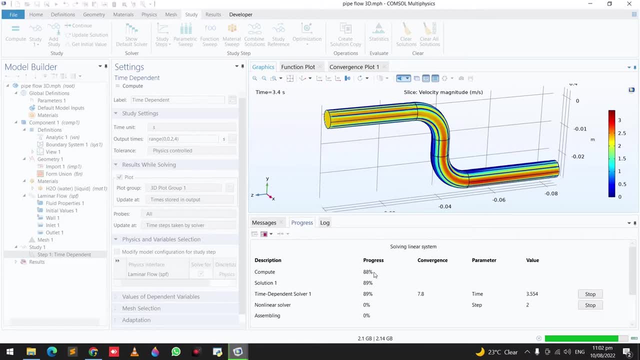 that we already solved for 3.4 second and we will go up to 4 second, and you and we will go up to 4 second, and you and we will go up to 4 second. and you can see the progress here it's going. 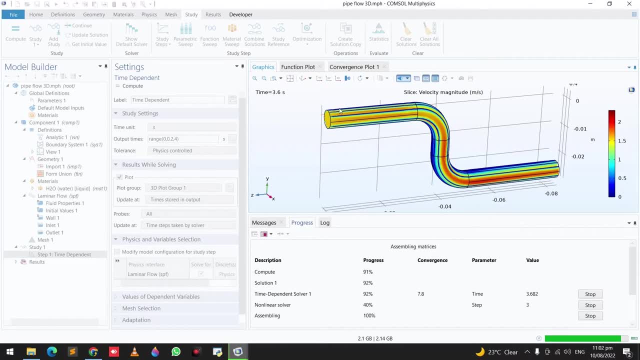 can see the progress here it's going, can see the progress here it's going very quickly. so once it's done and we very quickly. so once it's done and we very quickly. so once it's done and we can also see in the convergence floor is 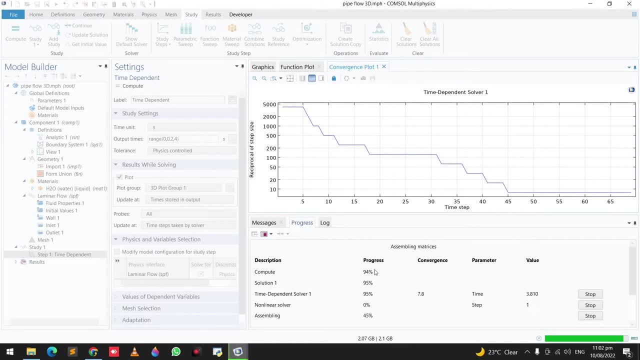 can also see in the convergence floor is- can also see in the convergence floor is going down and down. so we expect to going down and down. so we expect to going down and down. so we expect to simulate in coming few minutes and now. simulate in coming few minutes and now. 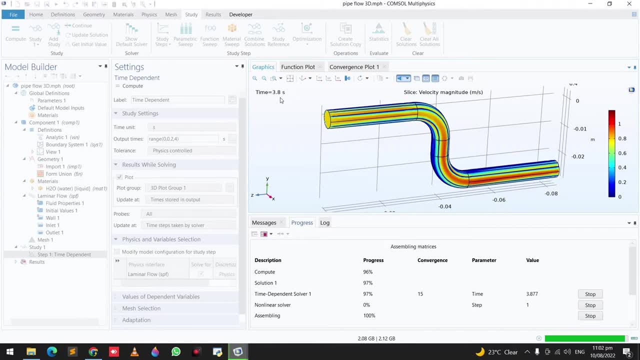 simulate in coming few minutes. and now you can see, here we almost reached to. you can see, here we almost reached to. you can see, here we almost reached to 3.8 second. and in the next step it will 3.8 second and in the next step it will. 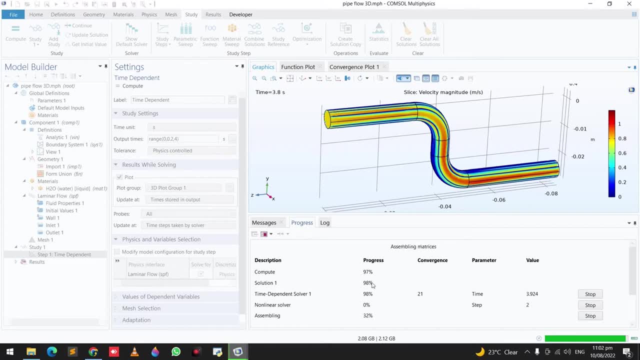 3.8 second and in the next step it will finish. so almost 95 sound percent of the finish, so almost 95 sound percent of the finish, so almost 95 sound percent of the simulation is completed. so once it's simulation is completed, so once it's. 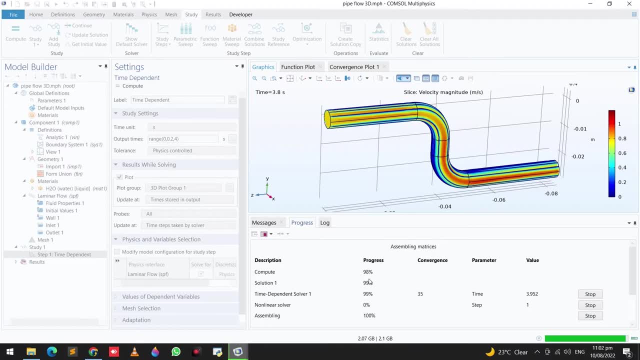 simulation is completed. so once it's done so, I'll show you that the details done so, I'll show you that. the details done so, I'll show you that the details of velocity profiles and how we can of velocity profiles and how we can of velocity profiles and how we can generate the animation. 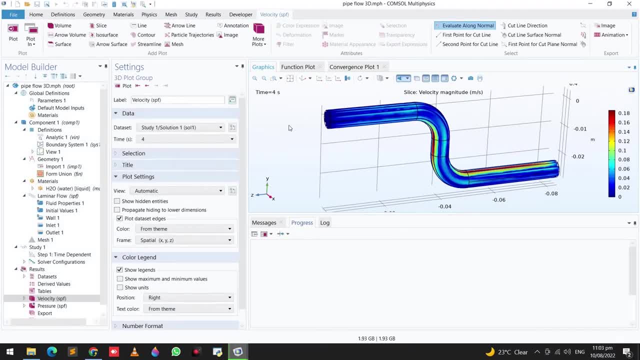 yes, now the simulation is completed. as yes, now the simulation is completed. as yes, now the simulation is completed, as you can see, here is being simulated for you can see, here is being simulated for you can see, here is being simulated for the four second, and we got a very nice. 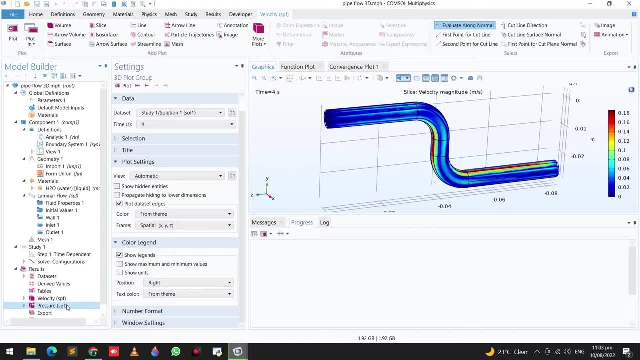 the four second and we got a very nice the four second and we got a very nice velocity profile and also the pressure velocity profile and also the pressure velocity profile and also the pressure profiles. so the problem with the profiles, so the problem with the profiles, so the problem with the velocity profiles. now slice is the number. 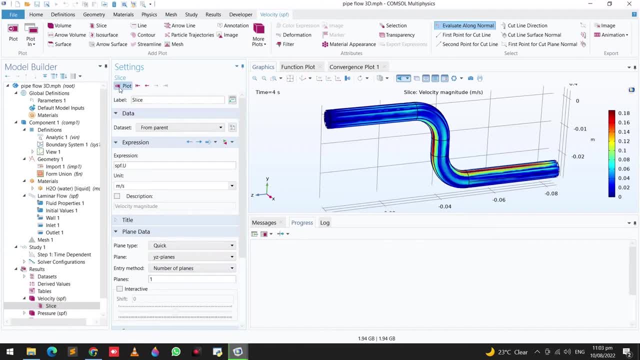 velocity profiles now slice is the number. velocity profiles now slice is the number of slices. so we can reduce it from five of slices. so we can reduce it from five of slices. so we can reduce it from five to one. and in plot and we can see here: 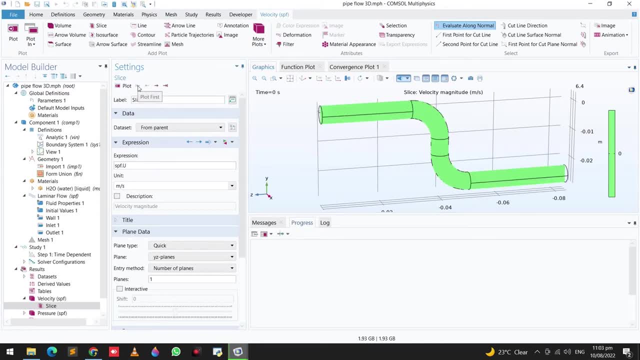 to one and in plot and we can see here- to one and in plot, and we can see here, and if you click here, so it will show us, and if you click here, so it will show us, and if you click here, so it will show us the first value, and if you click here, 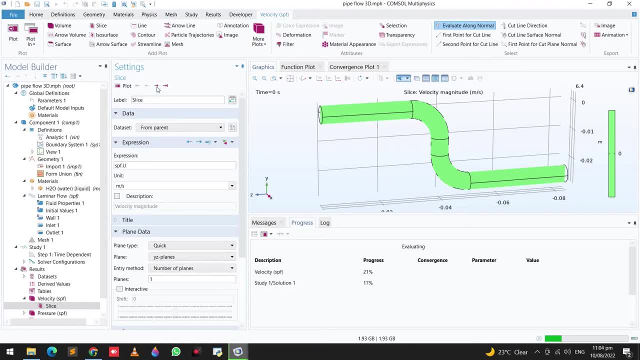 the first value and if you click here, the first value, and if you click here and show us with 0.2 step, so you can see, and show us with 0.2 step, so you can see, and show us with 0.2 step so you can see, here we can monitor the velocity. 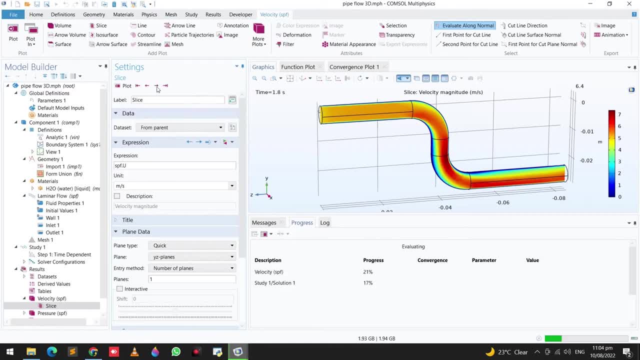 here we can monitor the velocity. here we can monitor the velocity profile at each time step. so what we can profile at each time step, so what we can profile at each time step, so what we can do is like we can include right click on, do is like we can include right click on. 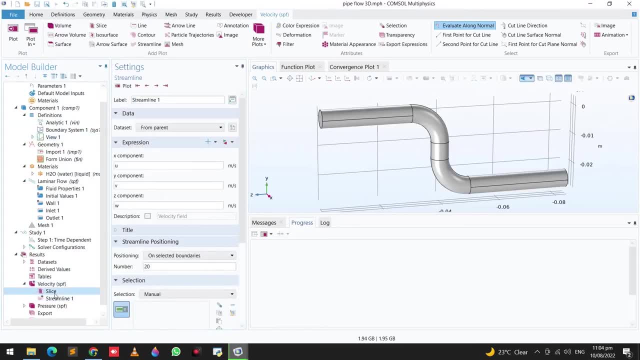 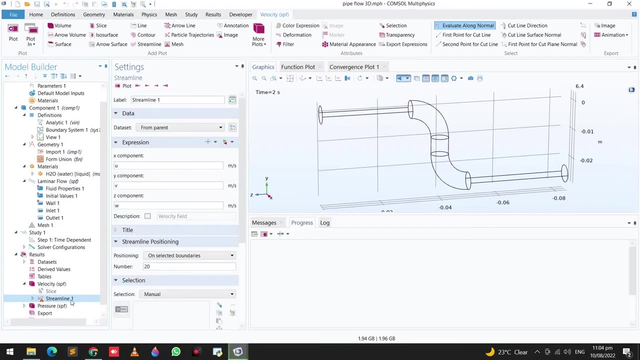 do is like we can include right click on the velocity and go to the streamlines, the velocity and go to the streamlines, the velocity and go to the streamlines and we can turn disable this slice and we can turn disable this slice and we can turn disable this slice function and we can select the inlet. 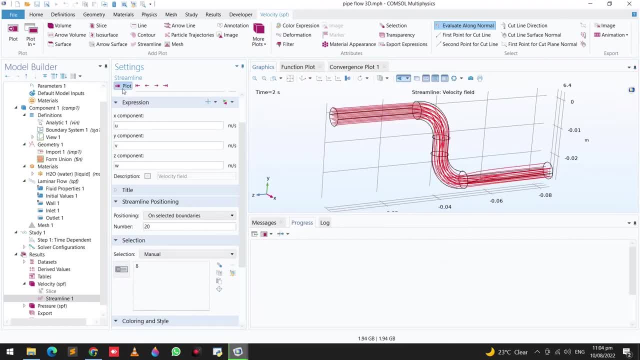 and we can select the inlet. and we can select the inlet, or this streamlines and, as you can see, or this streamlines and as you can see, or this streamlines and, as you can see, here we can increase the number of lines, here we can increase the number of lines. 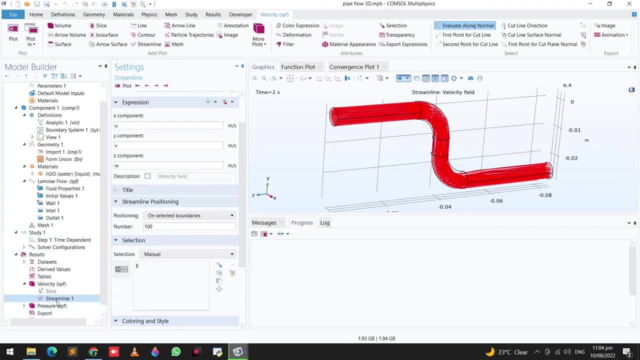 here we can increase the number of lines. let's see: or 50, 100, sorry, and then we let's see. or 50, 100, sorry, and then we let's see, or 50, 100, sorry, and then we can add the color. can add the color. 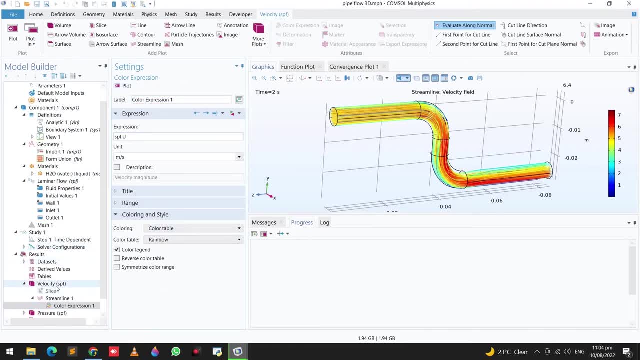 can add the color to this plot and you can see here, if now to this plot. and you can see here, if now to this plot and you can see here, if now, if we come and see how the velocity is, if we come and see how the velocity is. 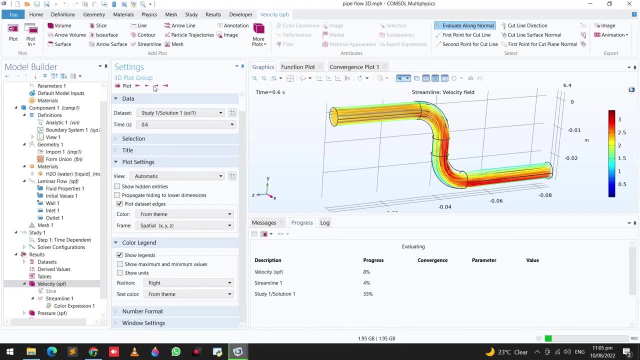 if we come and see how the velocity is lost profile is changing in streamline. lost profile is changing in streamline lost profile is changing in streamline function. so in the next step I will show function. so in the next step I will show function. so in the next step I will show you that, how you can generate animation. 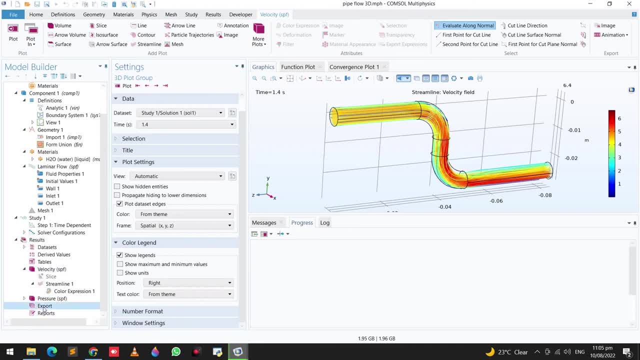 you that how you can generate animation. you that how you can generate animation for the same simulation. so go to the. for the same simulation, so go to the. for the same simulation. so go to the export and right click on the export and export and right click on the export and. 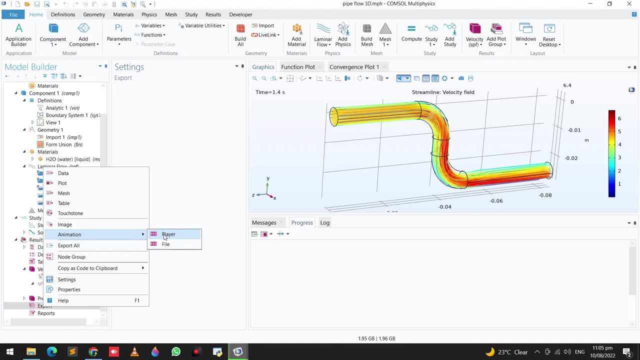 export and right click on the export and go to the animation and first reveal. I go to the animation and first reveal. I go to the animation and first reveal: I would like to see in the player mode and would like to see in the player mode and would like to see in the player mode, and then we will export the file. so, as you, 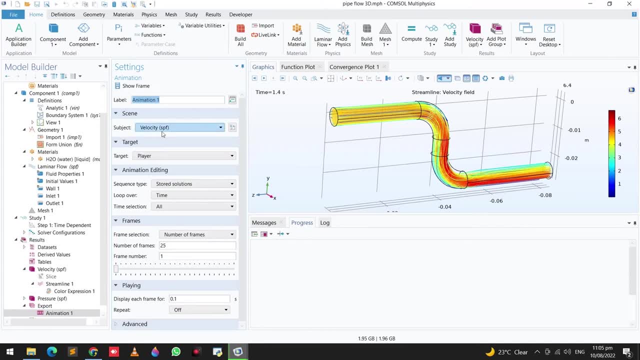 then we will export the file. so as you, then we will export the file. so, as you can see here the subject is lettered. can see here the subject is lettered. can see here the subject is lettered: velocity- so you want to see the velocity. velocity, so you want to see the velocity. 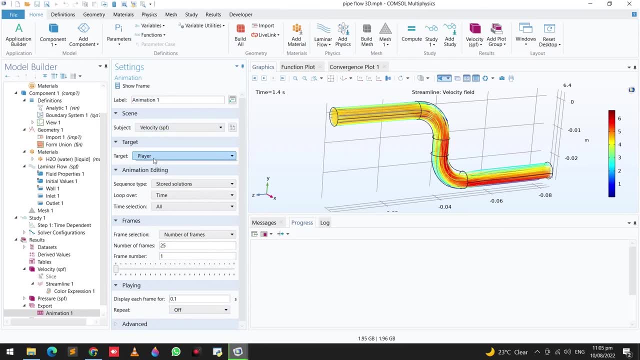 velocity. so you want to see the velocity profile and the target is player, so you profile and the target is player, so you profile and the target is player, so you can click on file and then concentrate, can click on file and then concentrate. can click on file and then concentrate the file either in gif, flash, avi, your 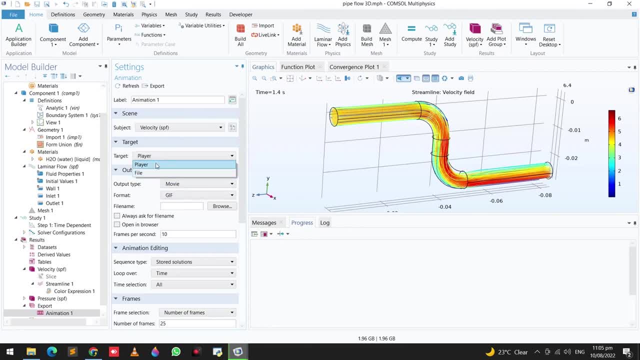 the file, either in gif flash avi. your the file, either in gif flash avi, your weapon. which extension do you want? so weapon, which extension do you want? so weapon, which extension do you want? so you click on the player and then we are. you click on the player and then we are. 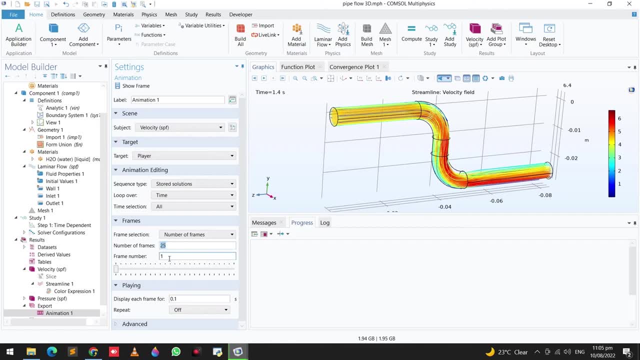 you click on the player and then we are going to. there's only there are 25 going to. there's only there are 25 going to. there's only there are 25 frames. so you can solve it for 25 frames. frames. so you can solve it for 25 frames. 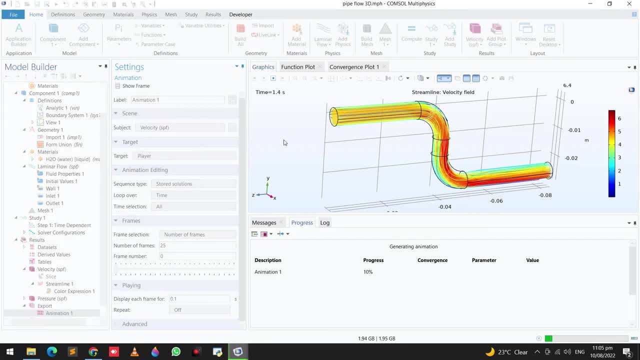 frames, so you can solve it for 25 frames, and then we will click on the generate, and then we will click on the generate and then we will click on the generate button so it will generate the animation button. so it will generate the animation button, so it will generate the animation and then we can see animation starting. 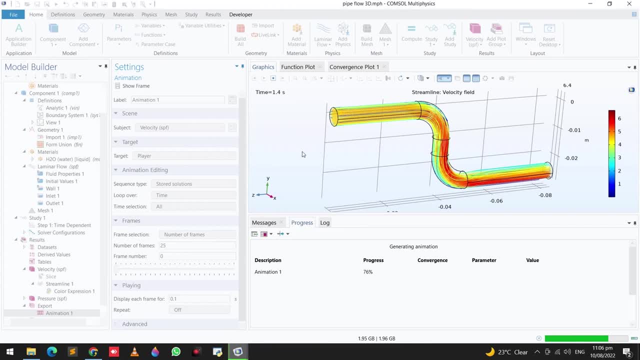 and then we can see animation starting, and then we can see animation starting from 0 second to 4 second. from 0 second to 4 second. from 0 second to 4 second. it will take few seconds, then it will. it will take few seconds, then it will. 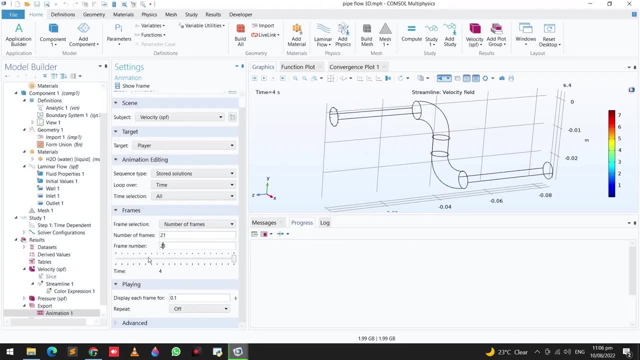 it will take few seconds. then it will automatically generate the simulation. as automatically generate the simulation, as automatically generate the simulation, as you can see here and what you can do to. you can see here and what you can do to. you can see here and what you can do to make. you can go to the repeat and then 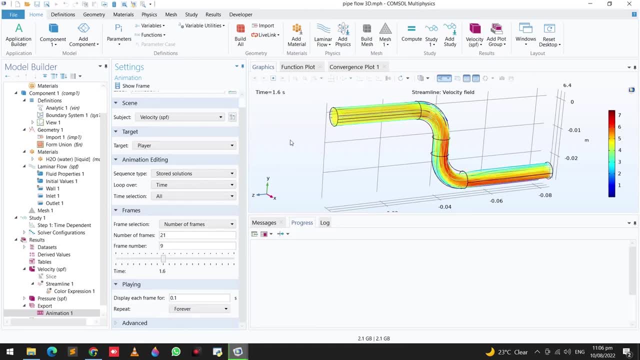 make you can go to the repeat and then make you can go to the repeat and then click forever, and then you can see the click forever and then you can see the click forever and then you can see the simulation going forever. you can see simulation going forever, you can see. 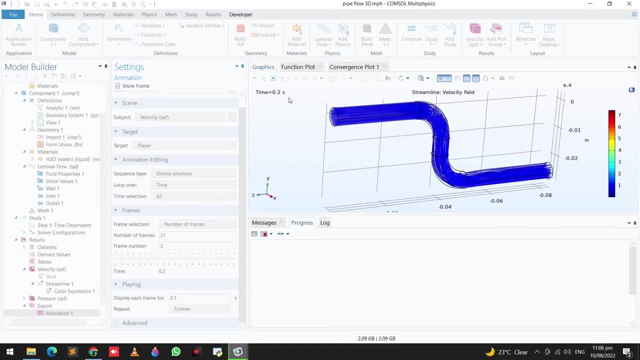 simulation going forever. you can see: here is starting from 0 second and going here is starting from 0 second. and going here is starting from 0 second and going to 4 second with the time step of 0.2 to 4 second with the time step of 0.2. 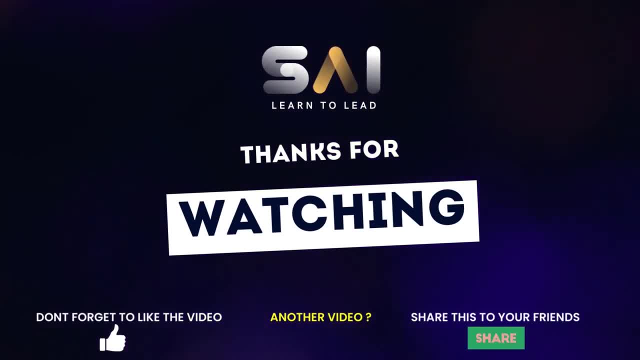 to 4 second, with the time step of 0.2.